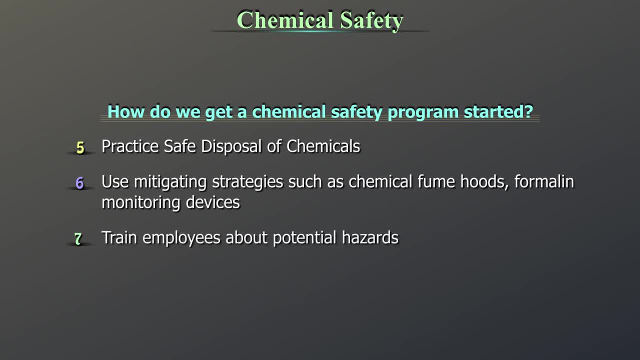 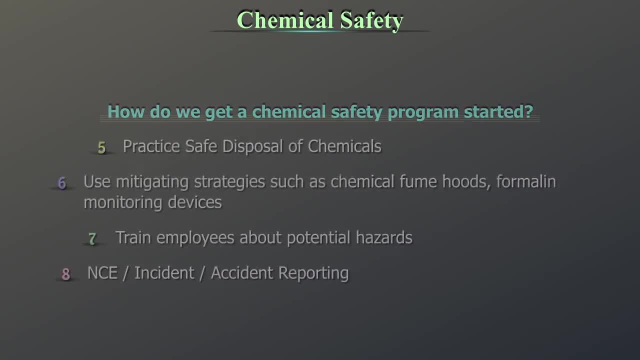 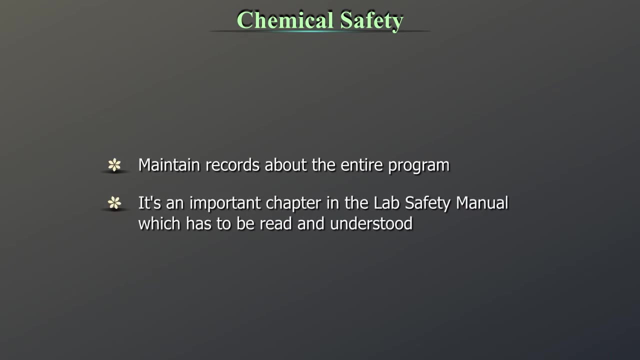 Is this what you want to do? Please let us know. Train employees about potential hazards, NCE or Incident or Accident Reporting. Maintain records about the entire program. This is an important chapter in the lab safety manual which has to be read and understood completely. 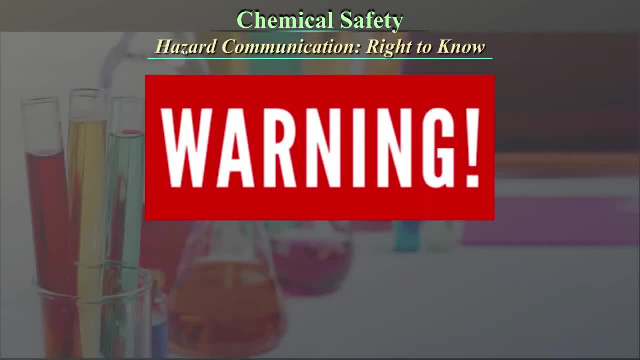 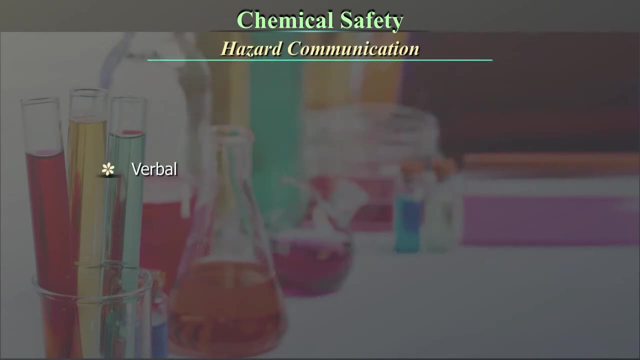 Hazard Communication. Right to Know. The lab staff have the right to know what chemicals they are using and how to use them, what are the risks and hazards and what precautions should be employed. All these are adequately indicated through several mechanisms like Verbal Visual Pictograms. 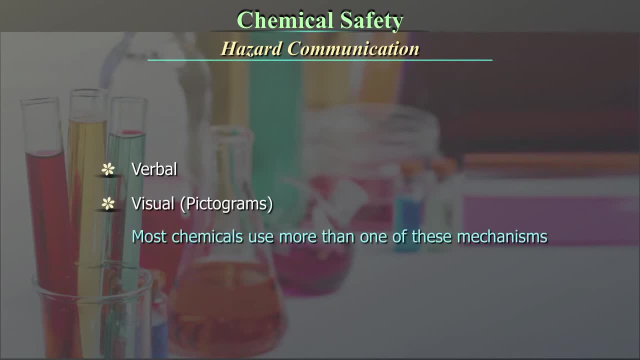 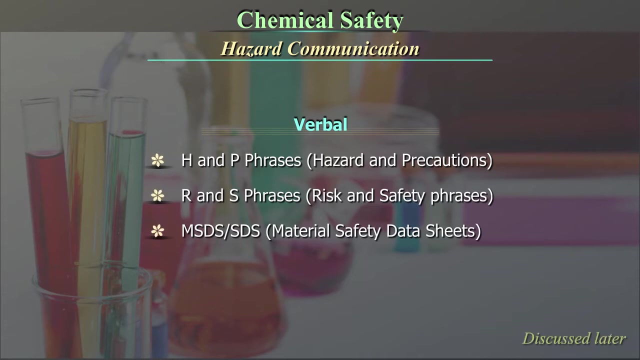 Most chemicals employ more than one of these mechanisms. Verbal H and P Phrases, Hazard and Precautions, R and S Phrases, Risk and Safety Phrases, MSDS or SDS Material Safety Data Sheets. The visual hazard communications are of three kinds. 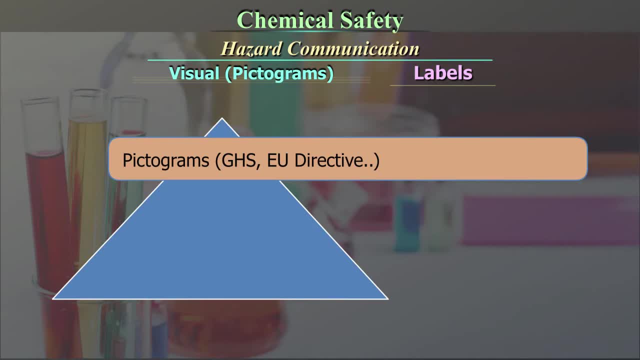 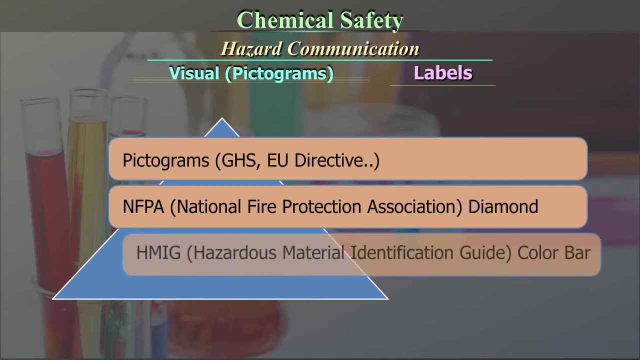 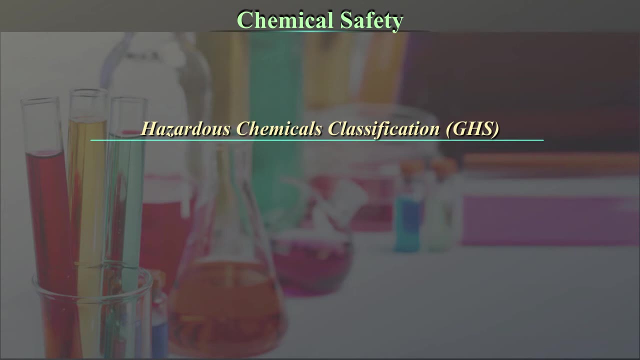 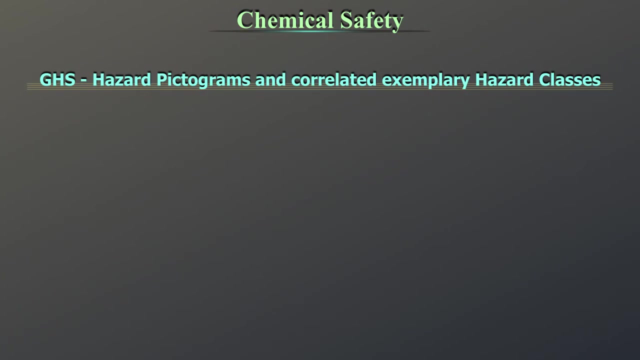 Labels, Pictograms, GHS, EU Directive, NFPA, National Fire Protection Association, Diamond, HMIG- Hazardous Material Identification Guide, Colour Bar. Hazardous chemicals are classified under GHS. Three main aspects of hazard are identified: Physical Health, Environmental. GHS Hazard Pictograms and the correlated exemplary hazard classes. 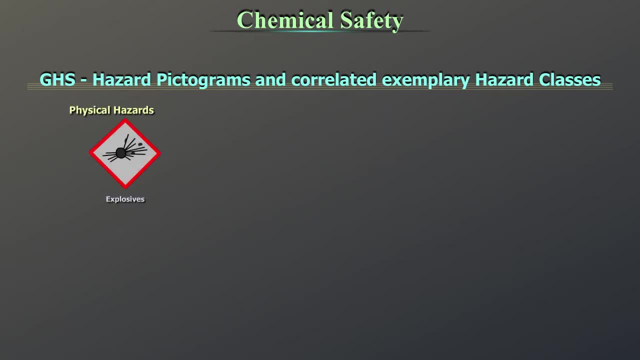 Physical Hazards: Explosives, Flammable Liquids, Oxidizing Liquids, Compressed Gases Corrosive to Metals. Health Hazards: Acute Toxicity, Skin Corrosion, Skin Irritation, CMR or STOT Aspiration Hazard. Health Hazards- Environmental Hazards. 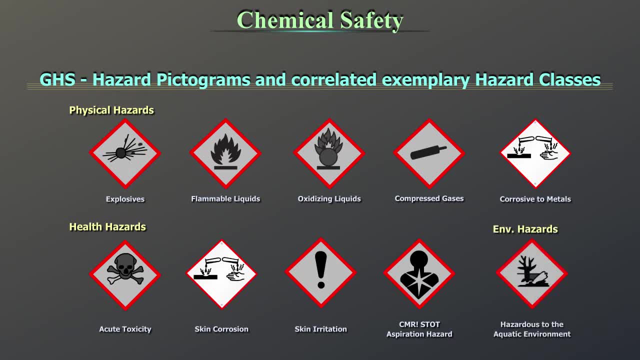 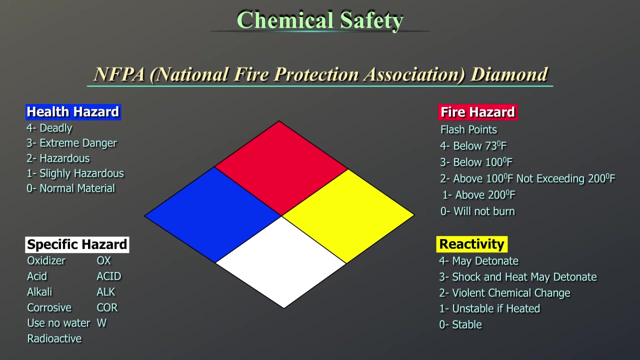 Hazardous to the Aquatic Environment. Note that CMR stands for Carcinogenic Germ Cell Mutagenic Toxicity Reproduction and STOT stands for Specific Target Organ Toxicity. The NFPA- Diamond, National Fire Protection Association. Another warning system is NFPA. 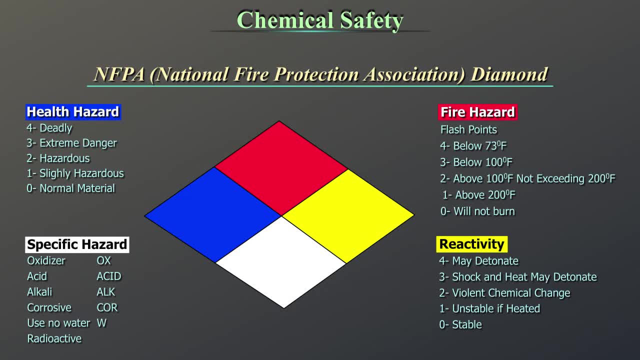 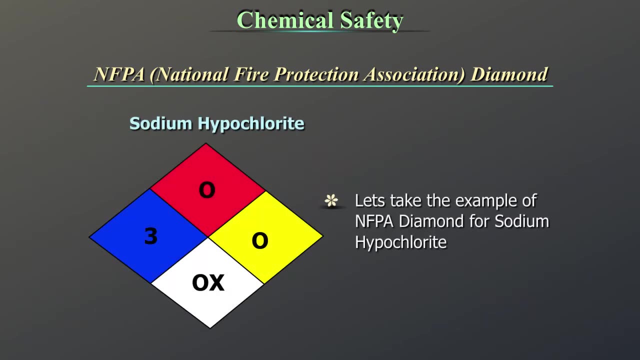 There are four diamonds within the one large diamond. Red indicates fire hazard. Blue indicating health hazard. White indicating a specific hazard. Yellow indicating reactivity. Let's take the example of the NFPA diamond for sodium hypochlorite. Sodium hypochlorite is a commonly used chemical in all labs. 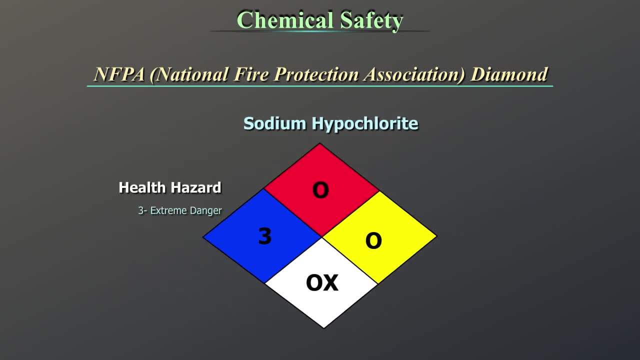 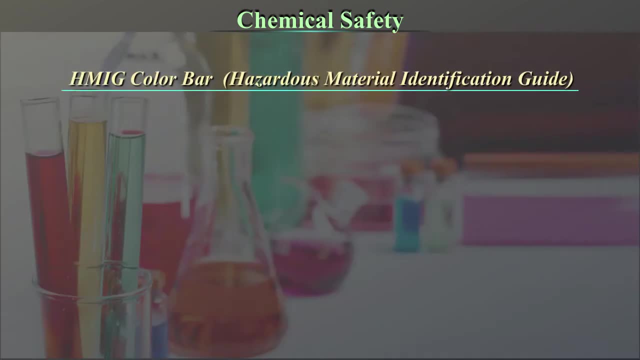 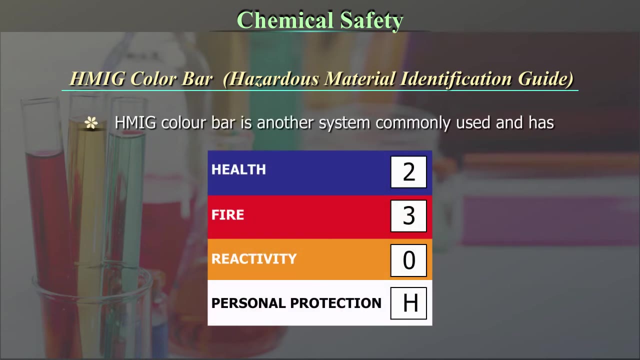 The NFPA says Category 3 for Health, 0 for Fire and Reactivity and oxidizing under specific hazard. HMIG Color Bar, or Hazardous Material Identification Guide. HMIG Color Bar is another system commonly used. It has blue for health, red for flammability. 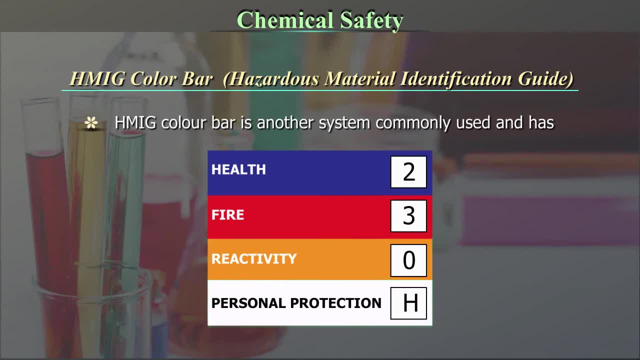 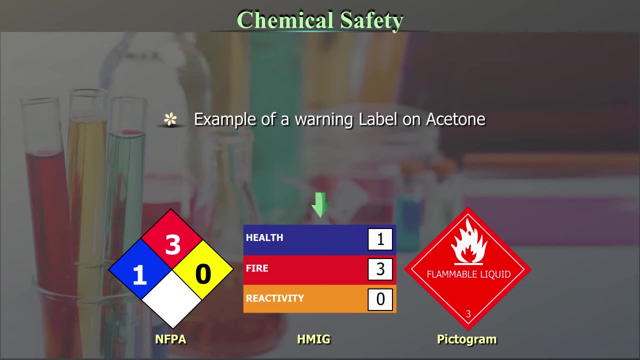 orange for physical hazard, ie reactivity, and white for personal protection, Fire and reactivity. both components of the physical hazards are separate. in this one Example of a warning label on acetone showing both NFPA and HMIG and pictogram is seen here. 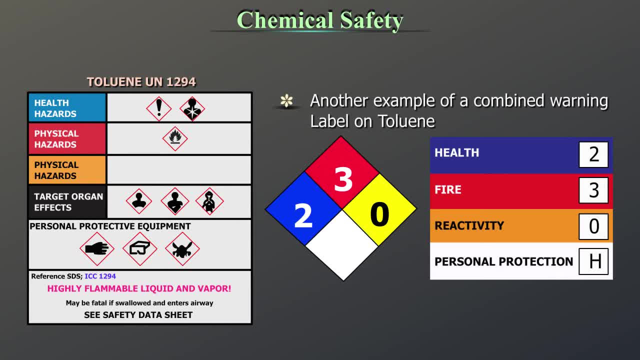 Another example of a combined warning label on toluene Fire is classified as a physical hazard, as in the case of GHS. Target organ effects are also specified. PPEs are illustrated. The right side shows separate NFPA and HMIG. 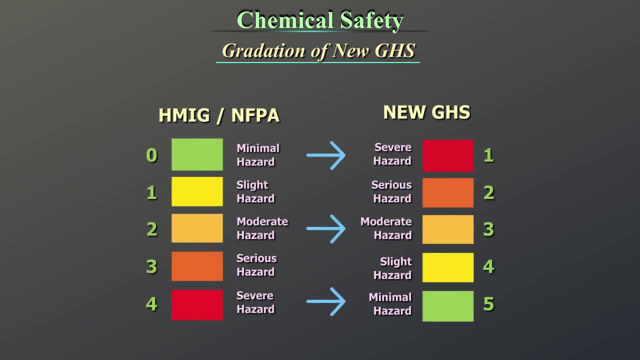 Gradation of the new GHG. The new GHS differs in its gradations from HMIG and NFPA. When HMIG and NFPA classifies green to red as 0 to 4, GHS classifies it in the other direction. green to red is 5 to 1.. 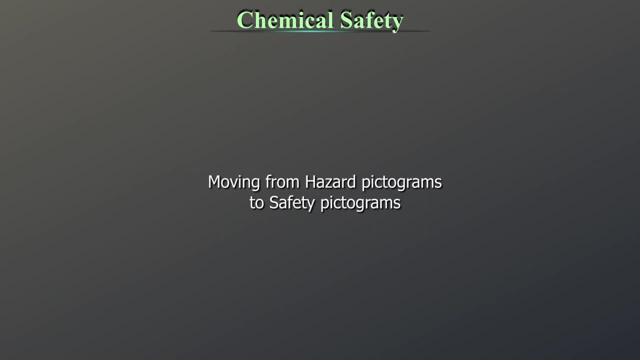 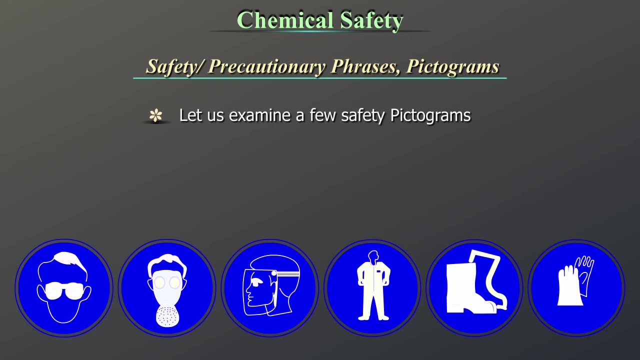 Moving from hazard pictogram to safety pictogram, Safety or precautionary phrases pictograms. Let us examine a few safety pictograms. You may see these cautions are not the same. They are based on different chemicals. You need to identify the use of these PPEs as indicated. 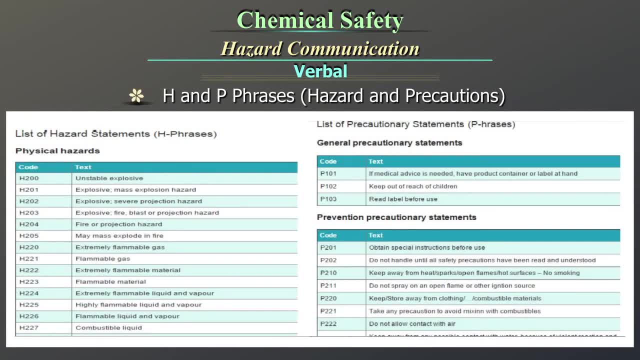 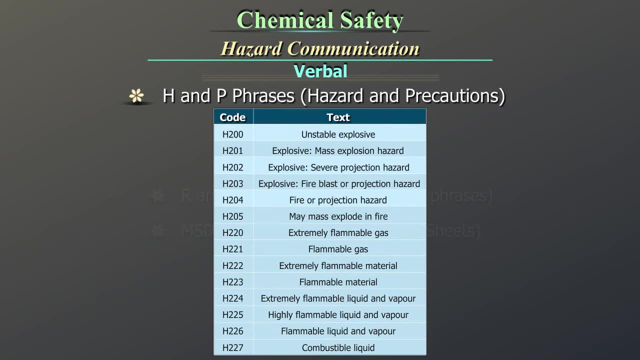 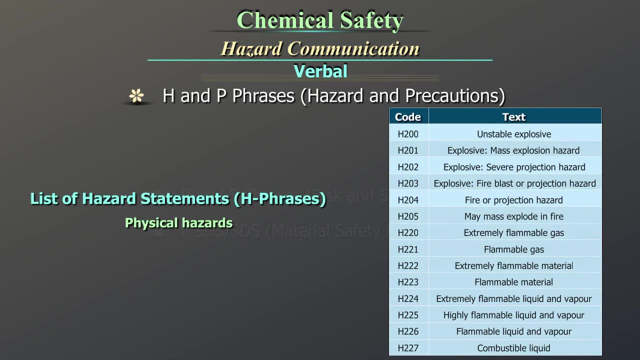 H and P phrases- Hazard and precautions. Now we can look at some H and P phrases, which is part of GHS. Here the list of H hazard phrases, H200 to H227, shows the code with its explanation. For example, H200 indicates unstable explosive. 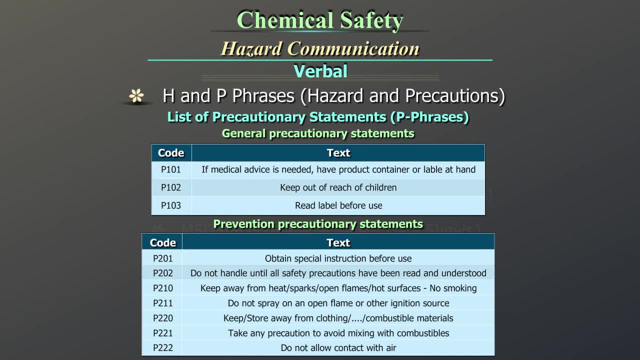 Similarly, there is a list of P phrases which are general and prevention precautionary statements. For example, P102 in general precautionary statements indicates keep out of reach of children And P201 in prevention precautionary statements indicates obtain special instructions before use. 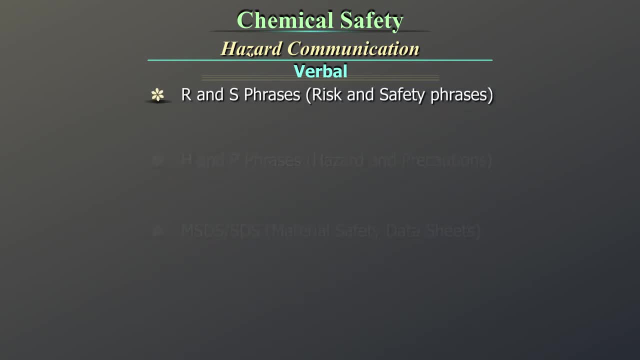 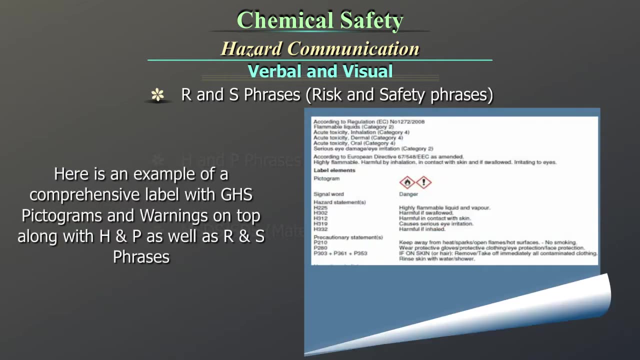 R and S phrases- Risk and safety phrases. This list shows the old system of R and S safety phrases. Here is an example of a comprehensive label with GHS pictograms and warnings on top, along with H and P, as well as R and S phrases. 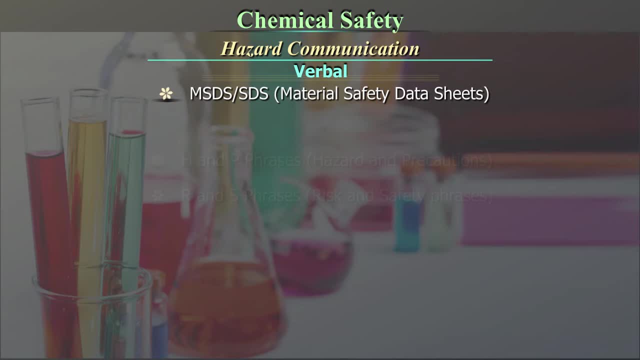 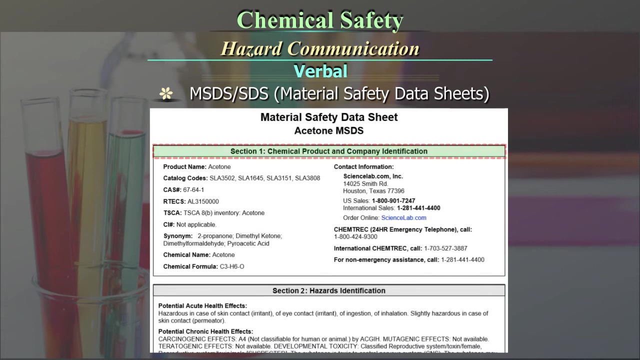 MSDS or SDS, material safety data sheets. This is another strong communication system. It is more detailed and gives much more information. Following aspects are addressed through a MSDS: 1. Identification of the substance or mixture and of the company or undertaking. 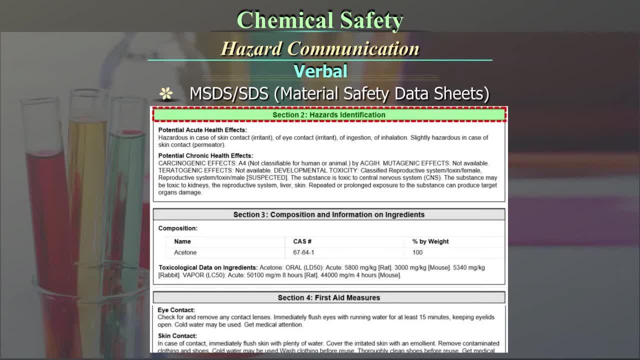 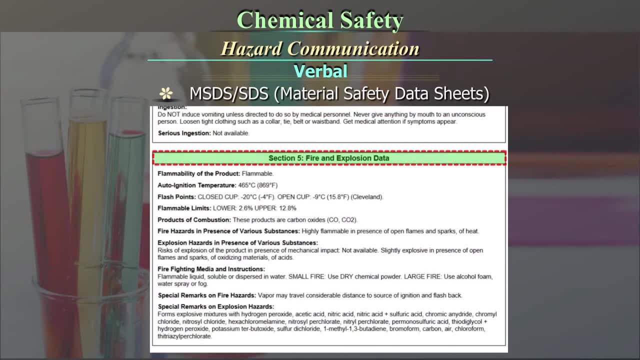 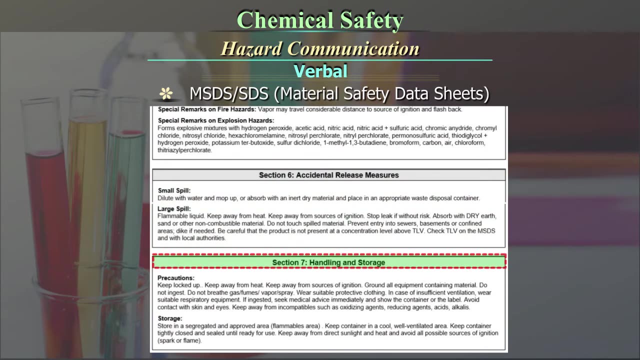 2. Hazards identification, 3. Composition or information on the ingredients, 4. First aid measures, 5. Firefighting measures, 6. Accidental release measures, 7. Handling and storage, 8. Exposure controls. 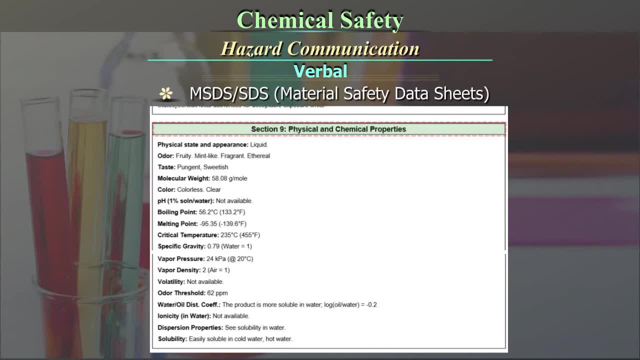 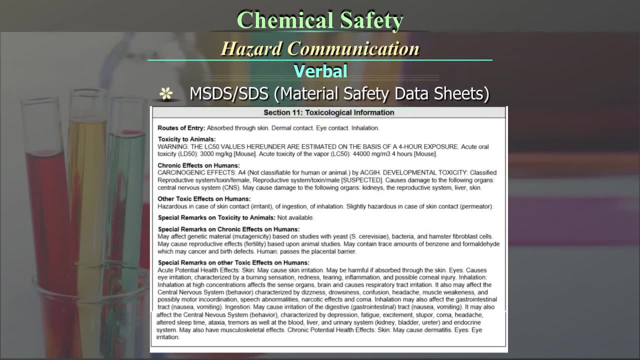 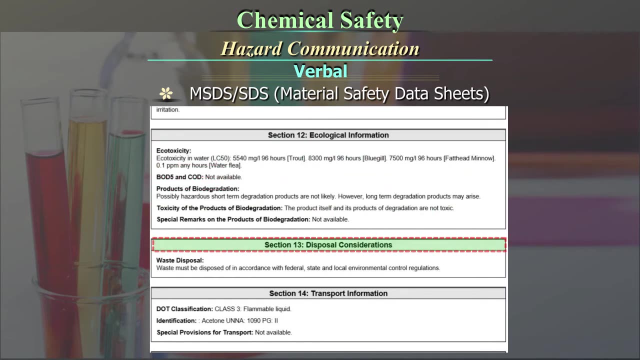 9. Personal protection, 9. Physical and chemical properties, 10. Stability and reactivity, 11. Toxicological information, 12. Ecological information, 13. Disposal considerations, 14. Transport information, 15. Regulatory information. 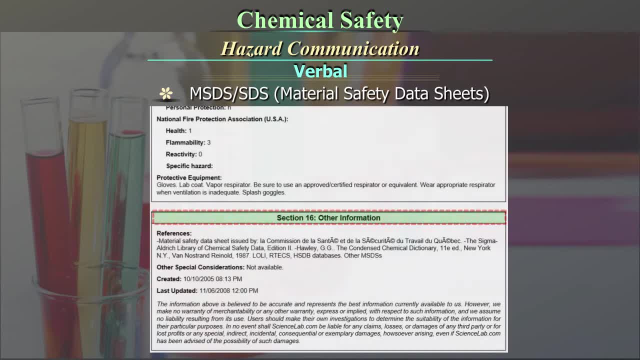 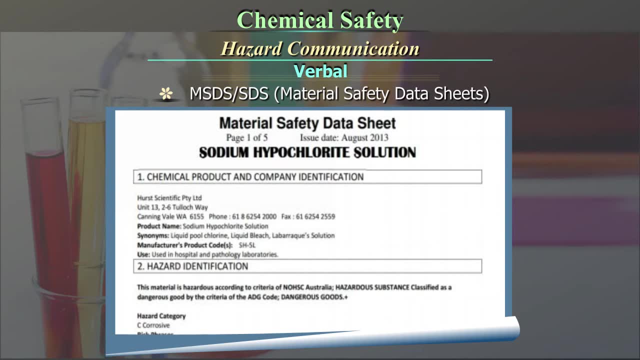 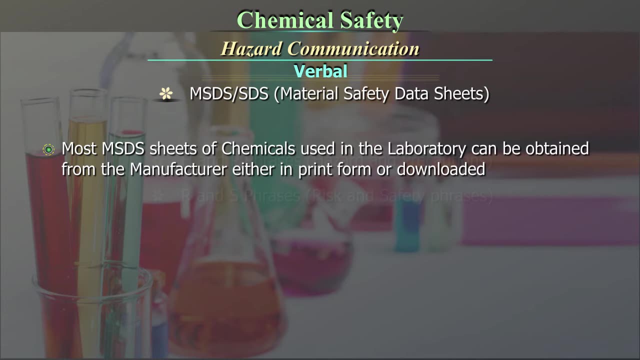 16. Other information. Here is an example of page 1 of MSDS of sodium hypochlorite. Most MSDS sheets of chemicals used in the laboratory can be obtained from the manufacturer either in a print form or downloaded. Ensure that the MSDS sheets are available at the point of use and are compiled in the documents of all chemicals and reagents used in the laboratory. 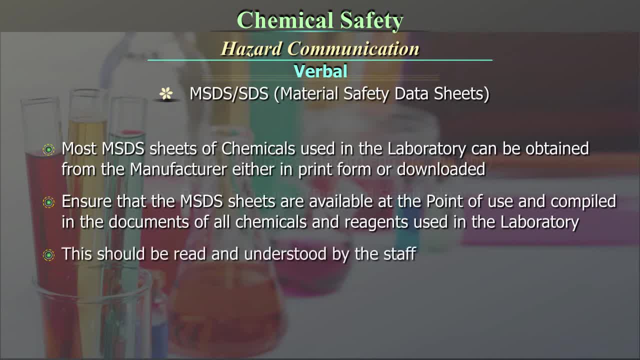 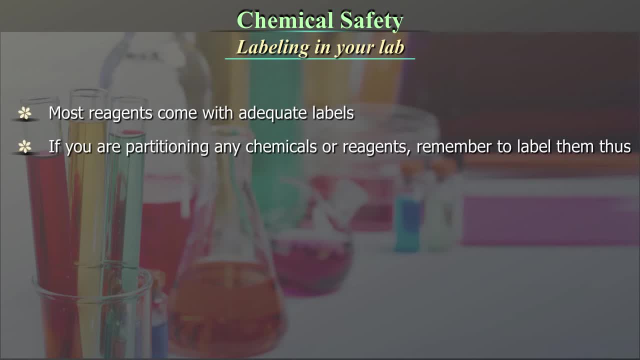 This should be read and understood by the staff Labelling in your lab. Most reagents come with adequate labels. If you are partitioning any chemicals or reagents, remember to label them thus: 1. The identity or contents of that container. 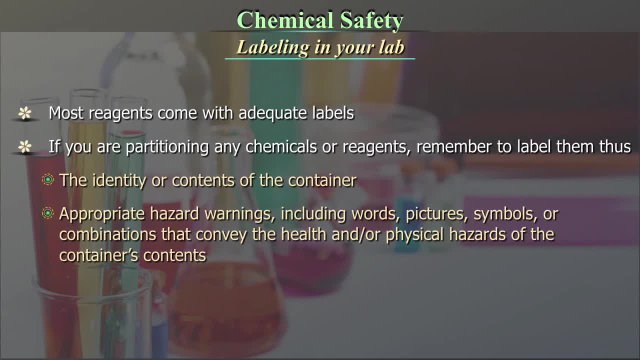 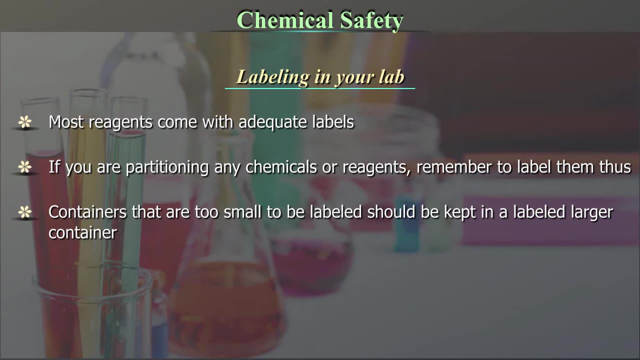 2. Appropriate hazard warnings, including words, pictures, symbols or combinations that convey the health and or the physical hazards of the container's contents. 3. The name and address of the chemical manufacturer and the emergency telephone number. Containers that are too small to be labelled should be kept in a large labelled container. 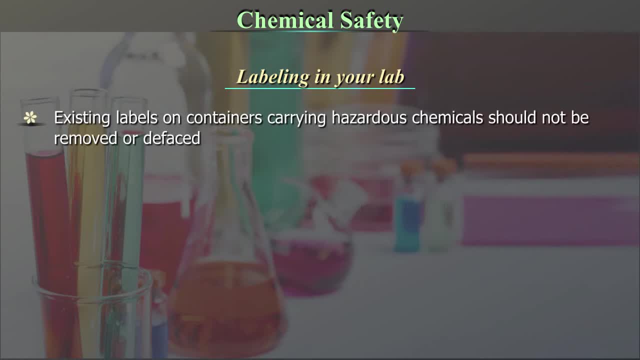 Existing labels on containers carrying hazardous chemicals should not be removed or defaced. Date of preparation and or the date placed in service and, where appropriate, the date of expiration, wherever warranted. Unlabelled: containers of chemicals should not be opened. Labels can be purchased or can be custom made by the laboratory. 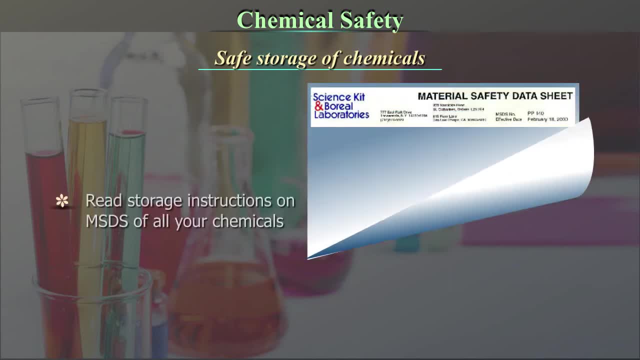 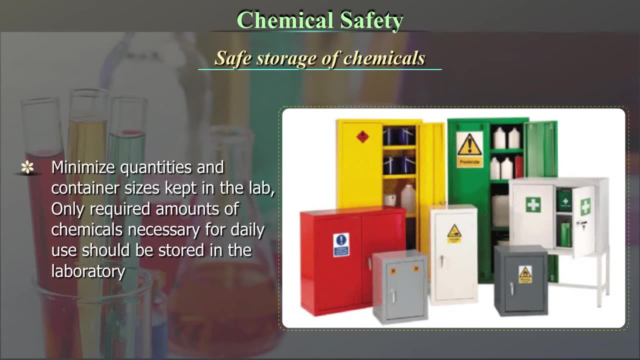 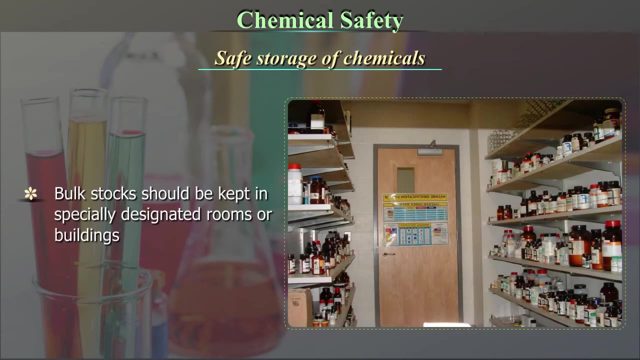 Safe storage of chemicals. Read the storage instructions on MSDS of all your chemicals. Minimize the quantities and container sizes kept in the lab. Only the required amounts of chemicals necessary for daily use should be stored in the laboratory. Bulk stock should be kept in specially designated rooms or buildings. 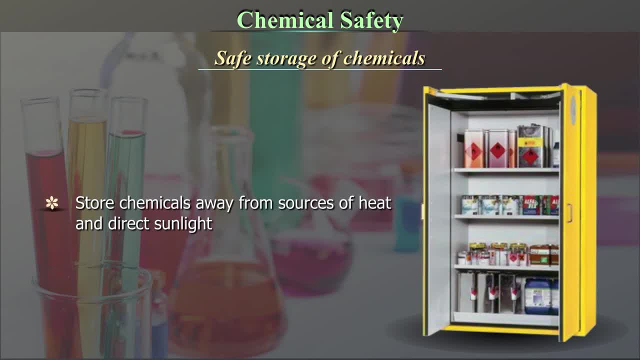 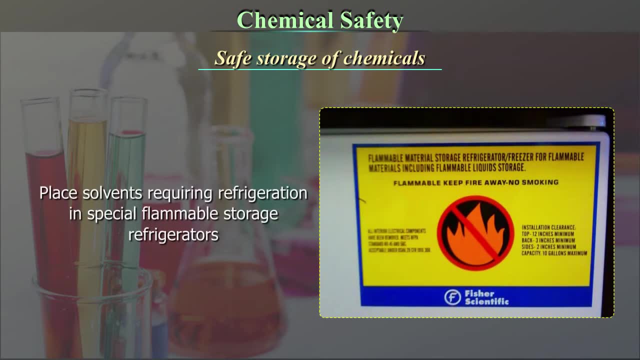 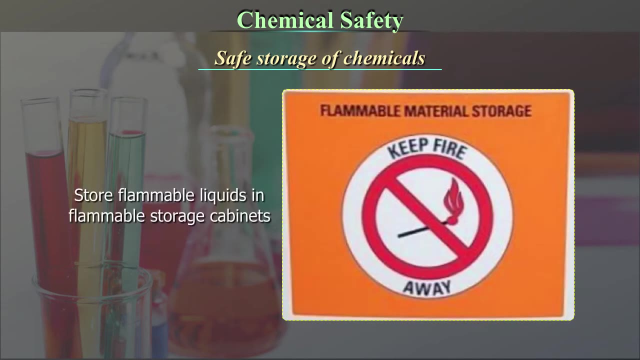 Store chemicals away from sources of heat and direct sunlight. Do not store hazardous liquids on shelves above eye level. Place the solvents requiring refrigeration in special flammable storage refrigerators. Store flammable liquids in flammable storage cabinets. Never pour flammable liquids down the drain because they can cause an explosion. 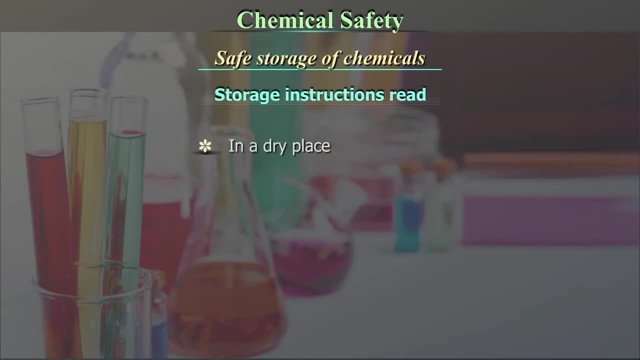 Storage instructions: read In a dry place, In a well ventilated place, In a closed container, Locked up In a corrosive resistant container Protected from sunlight. Do not expose to temperatures exceeding. Look at the labels Away from other material. Safe disposal: Dispose of unwanted chemicals promptly. Follow local regulations. 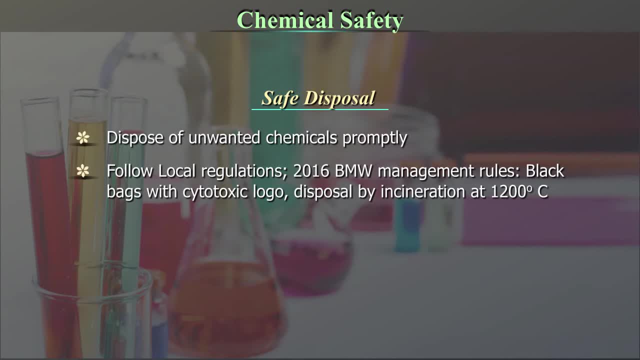 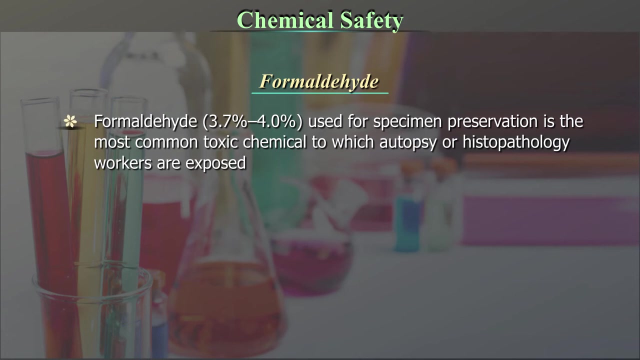 The 2016 BMW Management Rules: Black bags with cytotoxic logo. Disposal by incineration at 1200°C. Do not pour chemicals into the drain. Refer to manufacturer or supplier for recovery and recycling. Return to manufacturer for disposal. Formaldehyde- Formaldehyde- 3.74%, used for specimen preservation is the most common toxic chemical to which autopsy or histopathology workers are exposed. 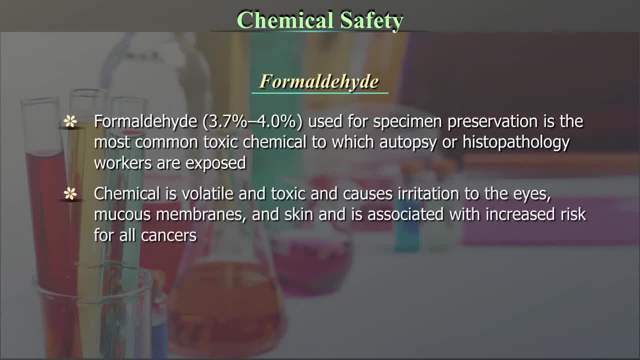 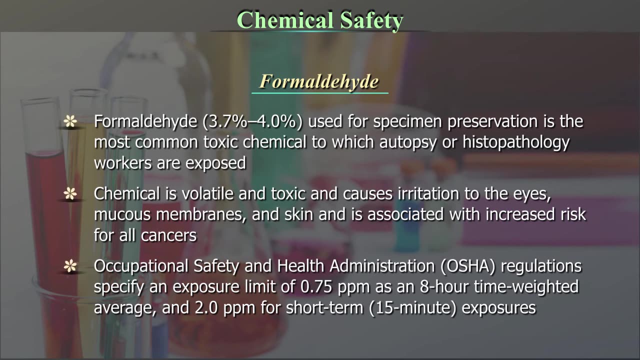 The chemical is volatile and toxic and causes irritation to the eyes, the mucous membranes and the skin and is associated with an increased risk for all cancers. Occupational Safety and Health Administration Regulations specify an exposure limit of 0.75ppm as an 8 hour time-weighted average and 2ppm for short-term exposures. 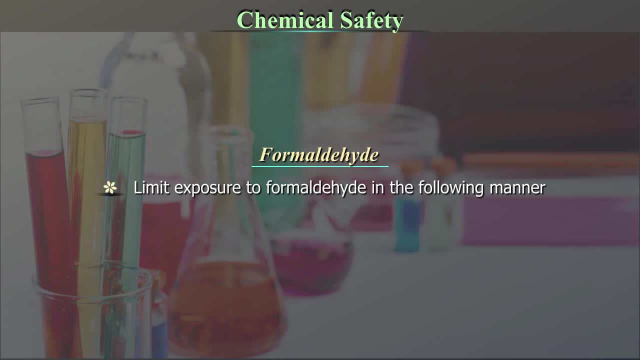 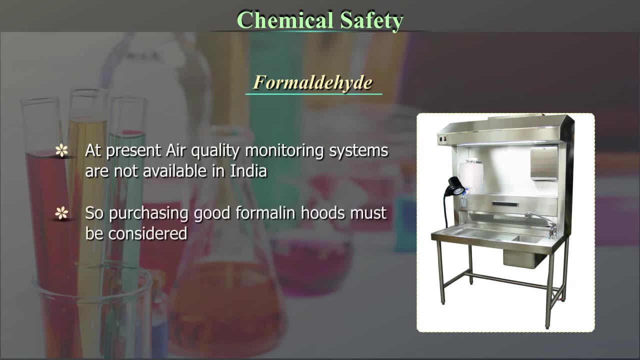 Limit exposure to formaldehyde in the following manner: At present, air quality monitoring systems are not available in India, So purchasing good formaldehyde hoods must be considered. The use of formaldehyde hoods reduces exposure to formaldehyde fumes. Cover all specimen buckets where the organs may be deposited for fixation. 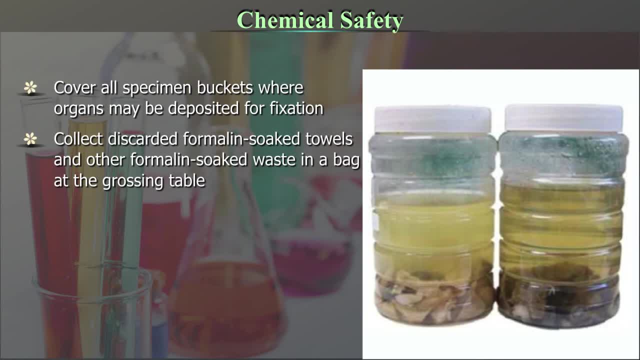 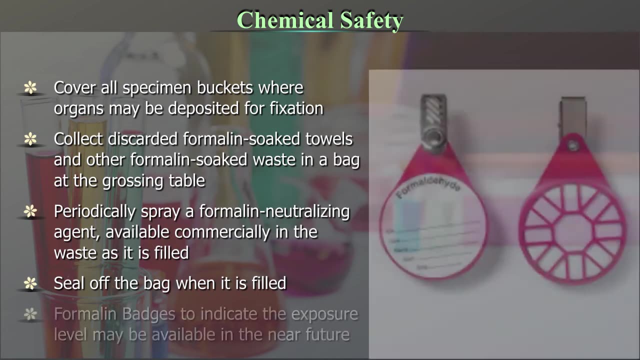 Collect discarded formaldehyde soaked towels and other formaldehyde soaked waste in a bag at the grossing table. Periodically spray a formaldehyde neutralizing agent available commercially in the waste as it is filled. Seal off the bag when it is filled. Formalin badges to indicate the exposure level may be available in the near future. 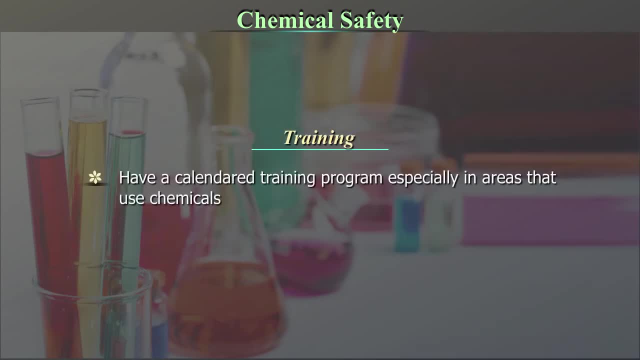 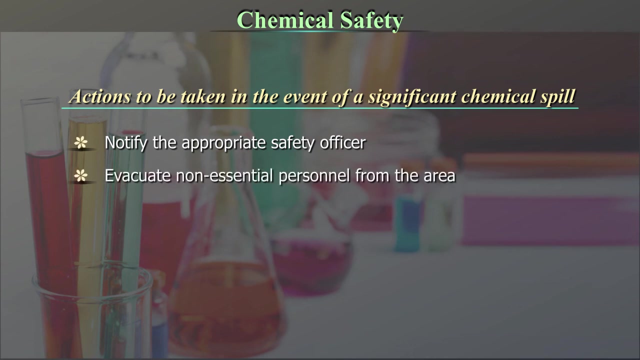 Training: Have a calendared training program, especially in areas that use chemicals, and have evaluation of that training. Actions to be taken in the event of a significant chemical spill: Notify the appropriate safety officer. Evacuate non-essential personnel from the area. Attend to persons who may have been contaminated. 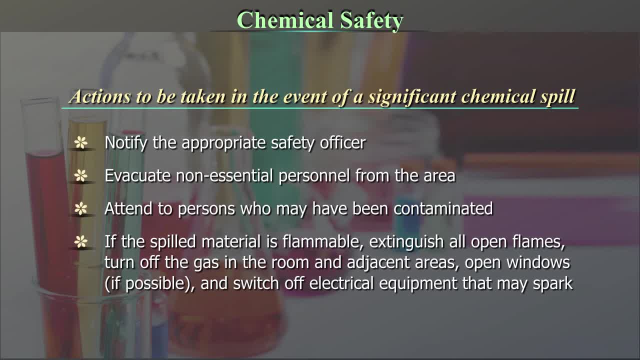 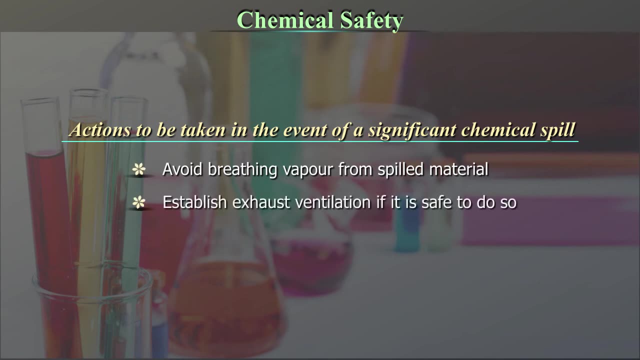 If the spilled material is flammable, extinguish all open flames. turn off the gas in the room and adjacent areas. open windows if possible and switch off electrical equipment that may spark. Avoid breathing vapor from spilled material. Establish exhaust ventilation if it is safe to do so.